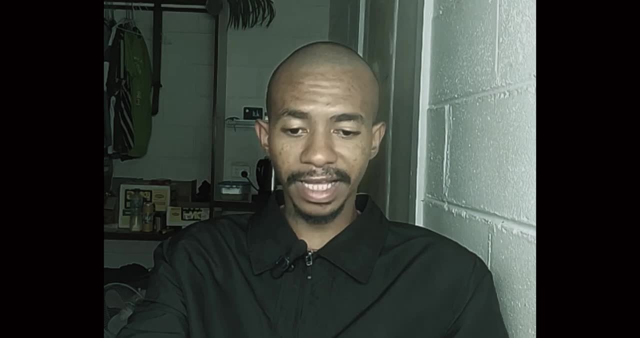 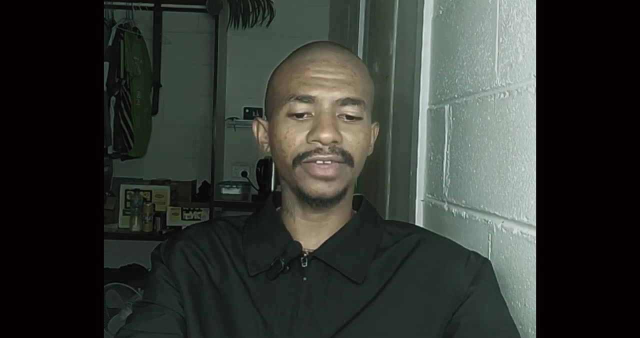 in terms of the livelihood of its citizens, and the latter being in a state of liability and prone to societal deterioration. In this study, we will discuss the definitions of dependency theory and the relationship between the two. What is dependency theory? Dependency theory explains the global economic system by describing how developing countries depend on developed countries for economic growth. according to GRU 2024.. Papua New Guinea is part of the underdeveloped countries of the global south, experiencing the hardships of being economically dependent. Many of these countries are unable to provide daily necessities for their citizens and are incapable of maintaining a progressive and sustainable economy. 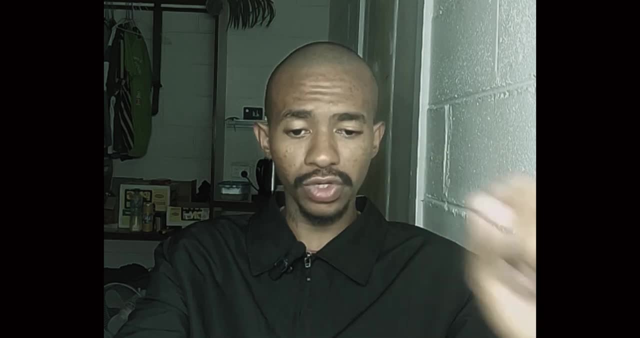 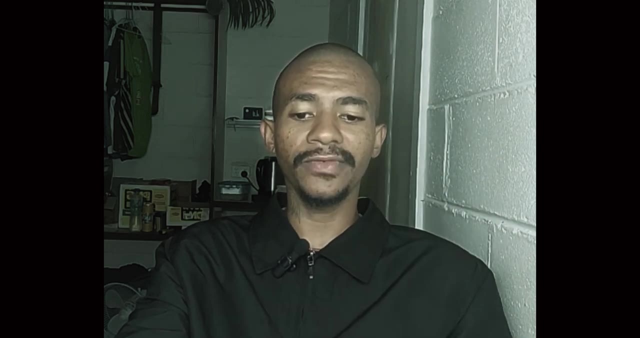 to meet the needs of their citizens. Many of these countries do not have the means to live the life-style of the modern world. This is due to the political and economic relationship between these two groups, As stated in the Lea 2000,. the world is divided into two main groups. 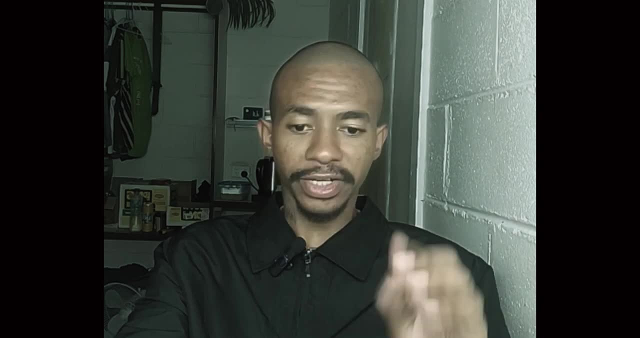 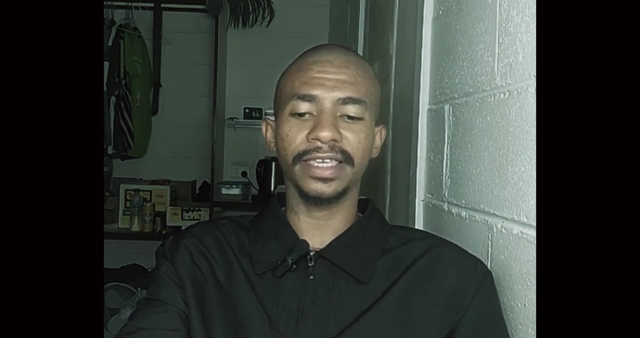 those who have economic power, the developed, the north, the center, the west or the metropoles, and their polar opposites. There are transnational corporations that act as agents that go around to peripheral countries, poor and exploit resources to transport to the semi-peripheral countries. 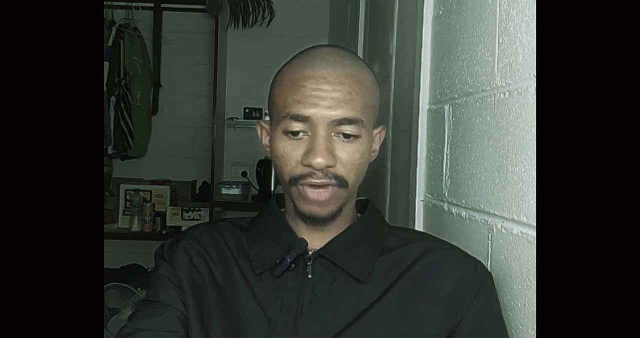 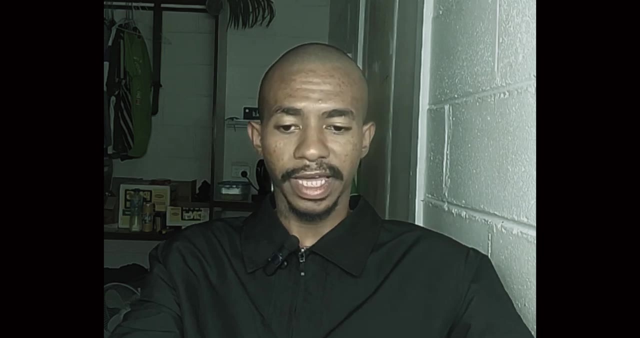 Core Rich countries, page 108.. These economic-powered countries then send back manufactured goods to the poor countries, and the cycle continues. It can be seen that all underdeveloped countries, including Papua New Guinea, find no choice but to invite foreign companies, eg gold mines and LNG projects. 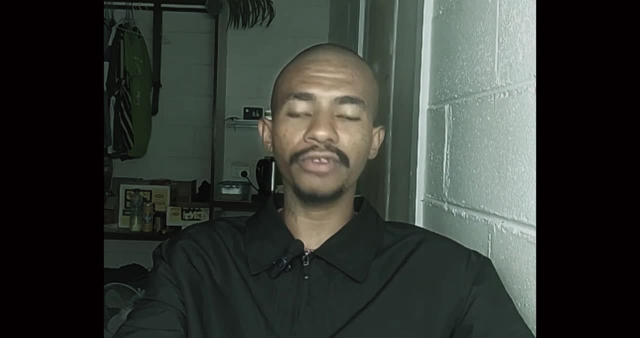 These companies are authorized to operate their activities through agreements from both their country of origin and the government of the country that they intend to run the operations in. In Papua New Guinea, the government owns everything that is six feet underground, The local citizens, who are mostly illiterate and depend wholly on the land for subsistence. 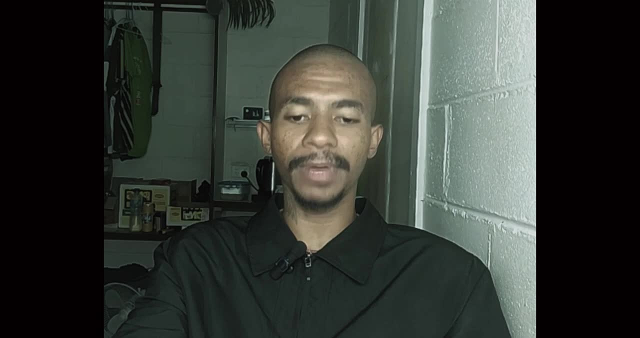 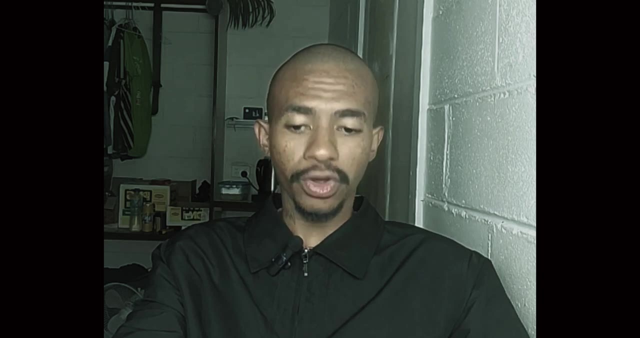 farming face deprivation. when large mining operations take place, The citizens are usually silenced with small amounts of compensation, commonly known as royalties. The countries in the Global North have formulated systems that they use towards the countries in the Global South in order to maintain their economic status. These strategies come in forms of loans, and a clear example is the various aids that other underdeveloped countries, including Papua New Guinea, receive from countries like USA, China and Japan. One hypothesis suggests that these are tactical approaches done to keep the peripheral countries dependent to the core countries. So, as the saying goes, the rich become richer and the poor become poorer. 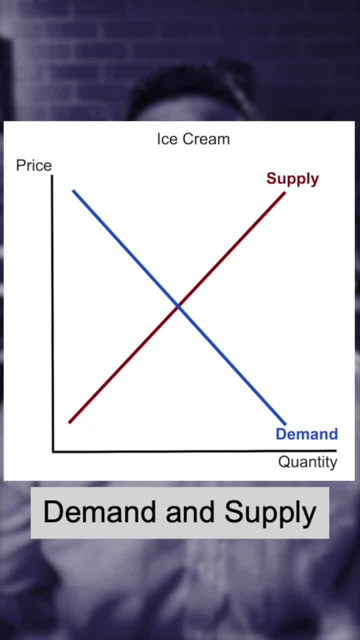 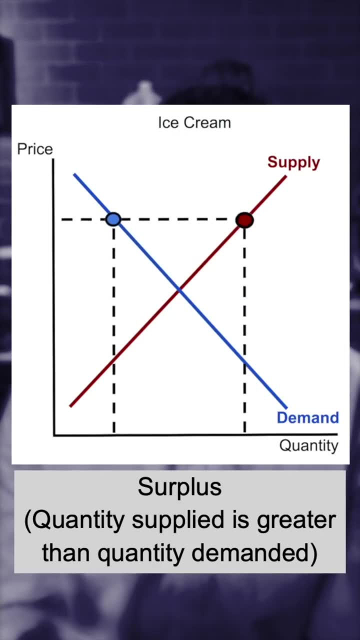 Okay, we've got demand, we've got supply. bam, put them together and you have the equilibrium price and quantity. But if the price was above equilibrium, the quantity supplied would be greater than the quantity demanded and we'd have a surplus. 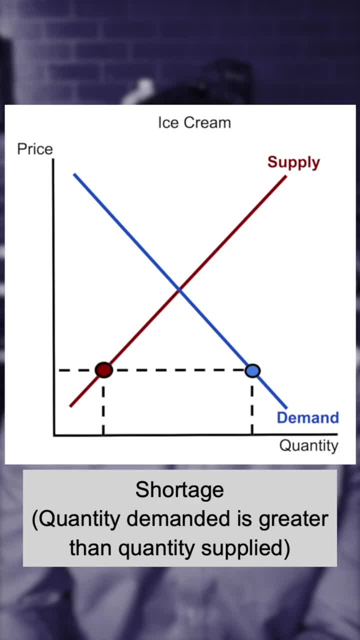 And if the price was below equilibrium, then the quantity demanded would be greater than the quantity supplied and we'd have a shortage. An easy way to remember that is: when the price is low, it's short. that's gonna cause a shortage.